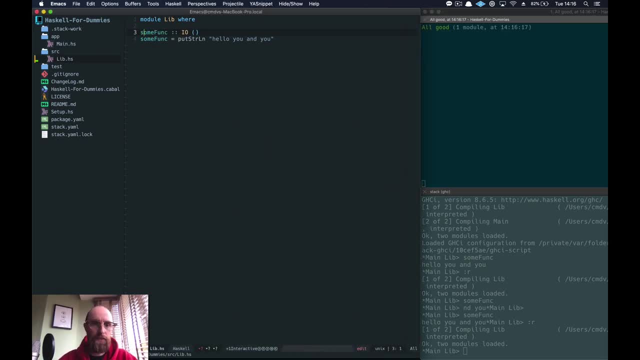 Uppercase is saved for types, So that would have to be lowercase, And then it's followed by these two colons, which indicates that it's going to be what type of what type it is. So in this case it's IO of unit, Then below that. 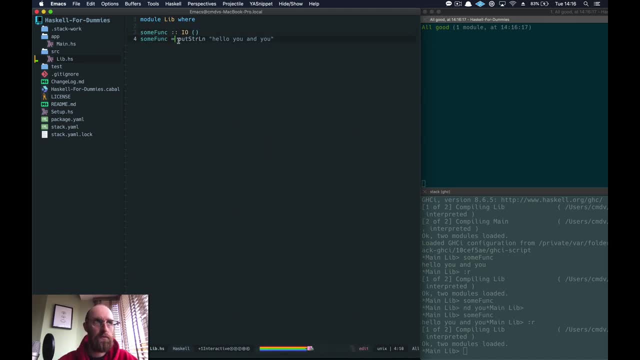 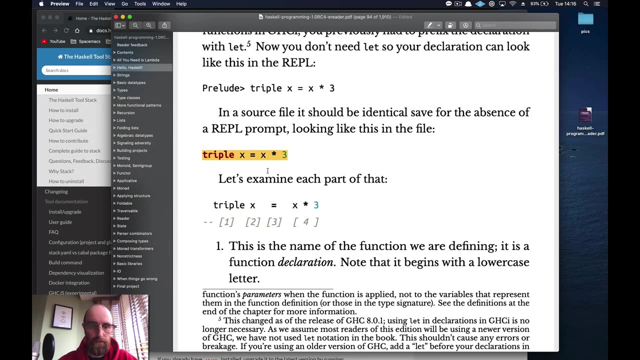 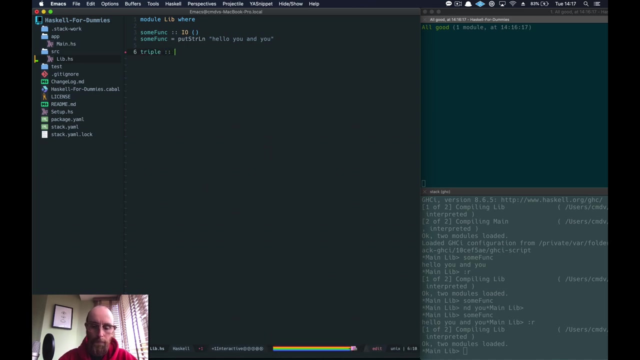 name your function again, and then you'd put an equal as to the content of the function, And in our instance it's put string line. Hello, you and you. But if we make something like a triple, we'll copy this example. Okay, so it does an int to int, So it takes an int. 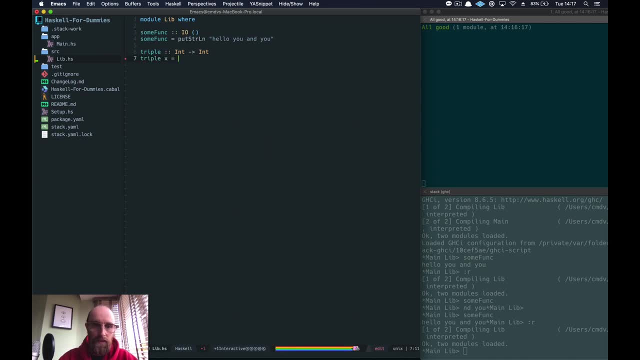 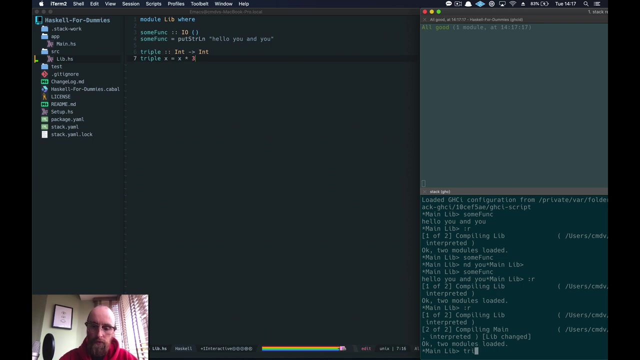 So let's call our int an x, And then we're going to say x times three because we want to triple it. So what we'll do now is we'll reload And we'll do triple one p And that does nine. So how is this working? So, essentially, it's replacing the x with a three. 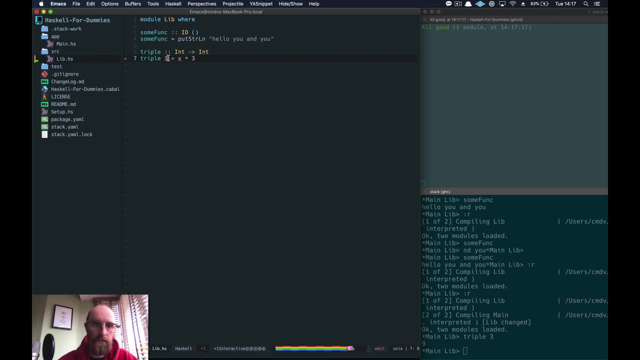 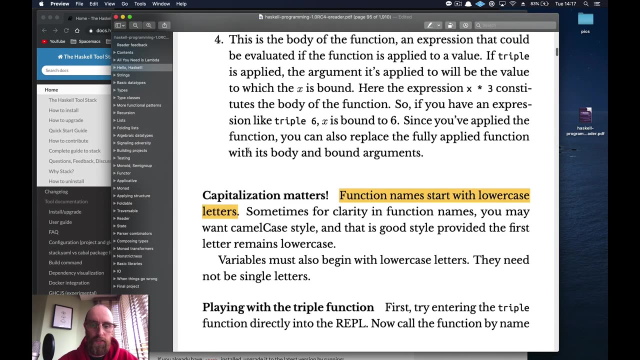 And it's doing like this: Okay, so that's replacing it, So you get three times three, which then equals nine. So that's a bit of an explanation of what's going on, And that's why I explained that the capitalization matters. The function needs to be in lowercase. 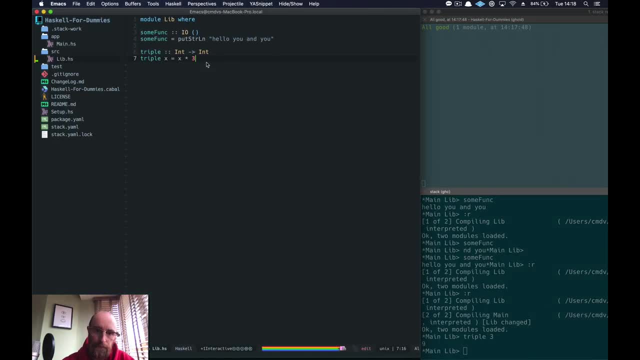 So so valuation. what it's actually saying is: these values won't execute until something comes in. When it's like this, it's in weak head, normal form, And then when it's evaluated, so when another int comes in- in our case it was another three- then it's in normal form because it's been. 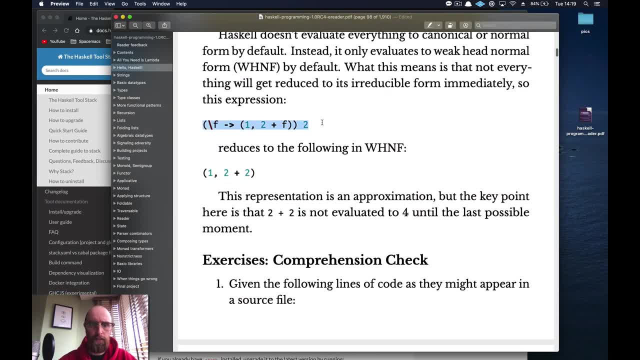 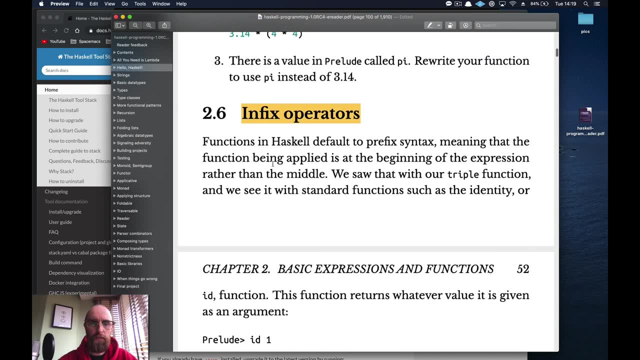 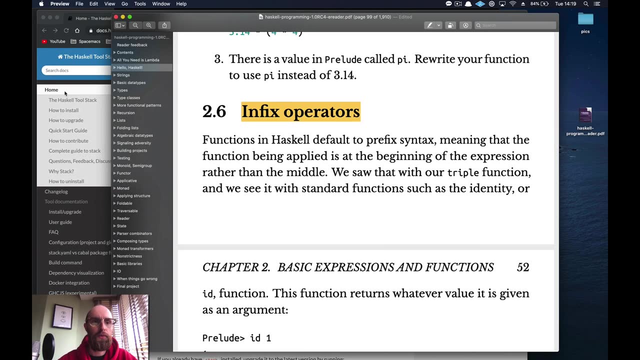 evaluated, so we'll ignore that for now. i'll explain that later what the backslash is. so infix operators. so this is a good one. now what you can do is if you see, oh, actually a good example of showing that is sometimes if you want to search, like before we were looking for. 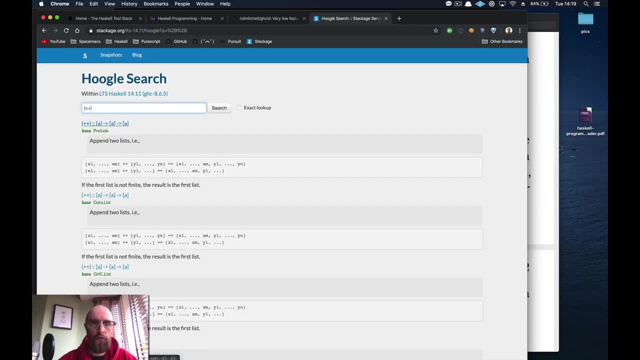 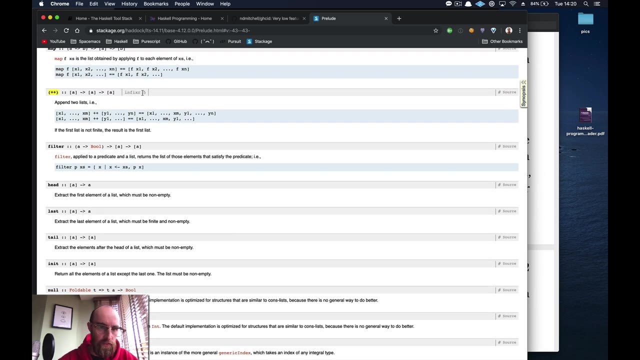 plus plus. so if you type plus plus and search for it, that'll work. but generally can you see it's wrapped in parentheses. so if i press enter, there we go and that's what an infix is. so let's have a look there and what this means. here we go. infix r of five and what this essentially means. 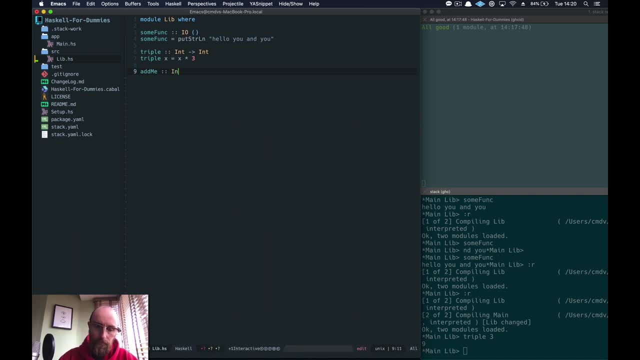 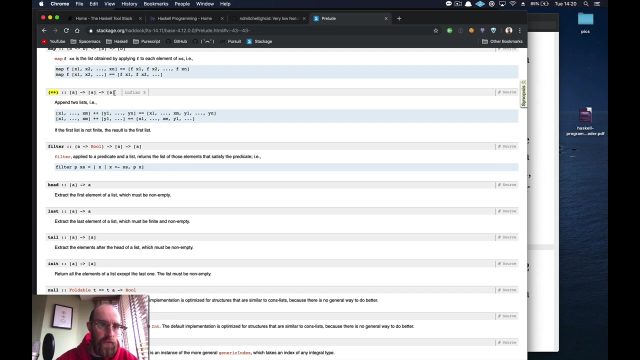 is this: add me- that'd be an int to an int- and add me, or take an. take an a and it'll be a plus 10.. okay, so you can do it like that, but you can also do it like this, because a, in essence, it takes a list of a, a list of a, and returns us an a. so, as 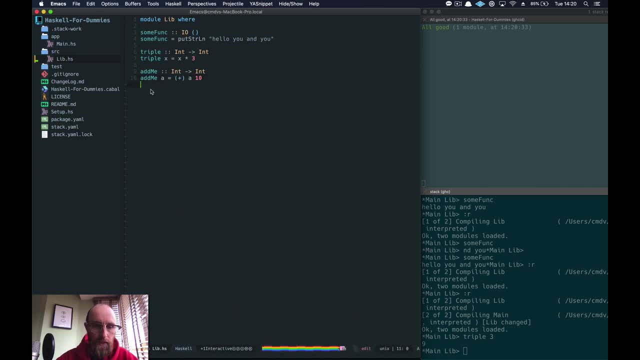 you can see. what we're saying is as when you're using add me- let's give you a little example. so let's reload that. add me four. that should give us 14.. okay, so what it's saying is that value int is our four and then, in that case, this first value. 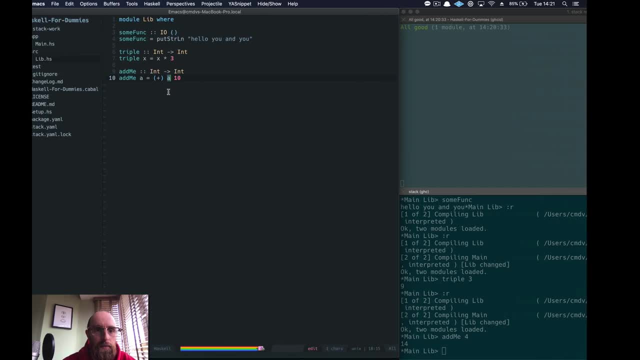 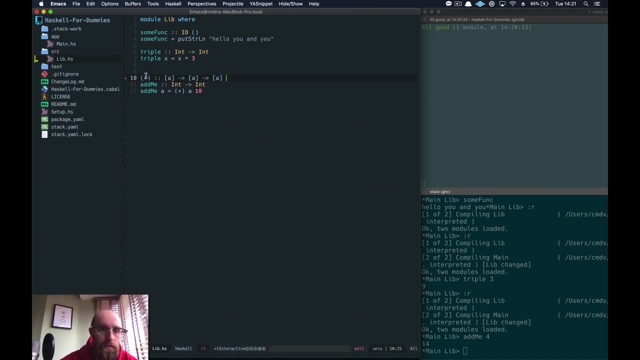 is. so let's, let's get the types actually, because that make a bit more sense and we'll do. plus is that type. i'll hide that away. so the a will be this and then the 10 will be this, and we'll explain in terms, because you 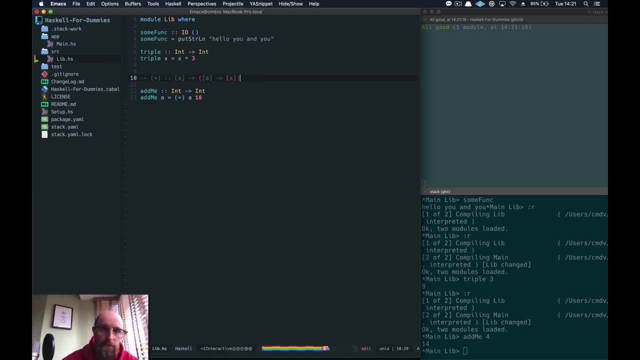 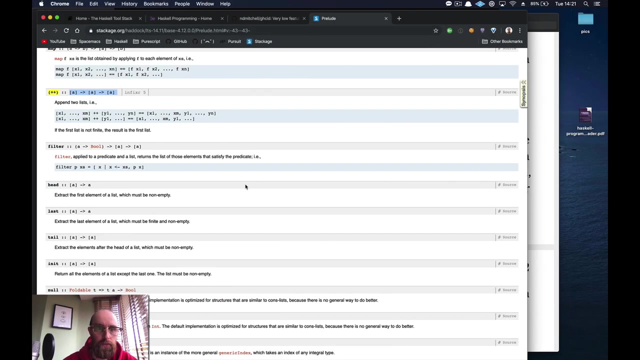 later i'll explain that it actually also becomes this, but that gets a little explained why it becomes like that. but if we just take it like this, so that's what an infix is- you're essentially saying that you can use this in this way also. there's alternate ways to use that. 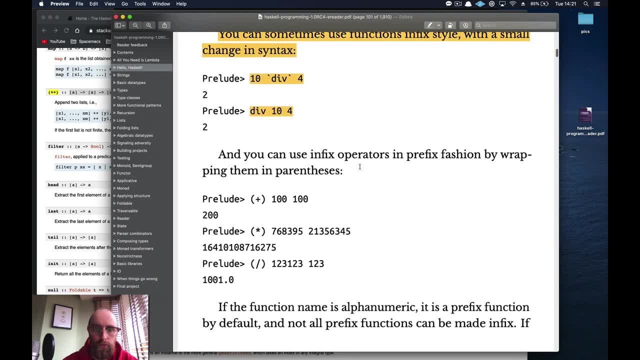 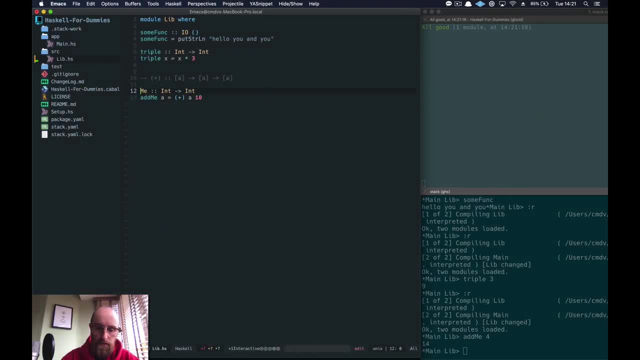 okay, so that's the infix operator, and let's have a little look at an example. this is a good one, dividing, so we'll call it div me. actually, let's create a new function: div me. it takes an int and it returns an int, and there's our int, and then we'll do a, and this is another way to do it. 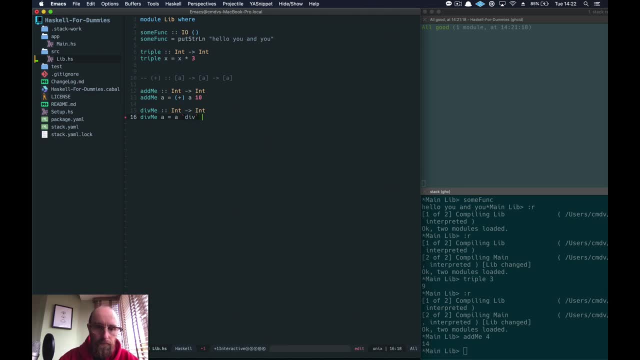 way to infix back. tick, and we'll divide by two. div me, let's call it, let's call this. div me by two. that's a bit better, isn't it? div me by two: give it an a div two. so let's have a little refresh, let's get the type of div, so it's. let's ignore this little part for now. it takes an, a. 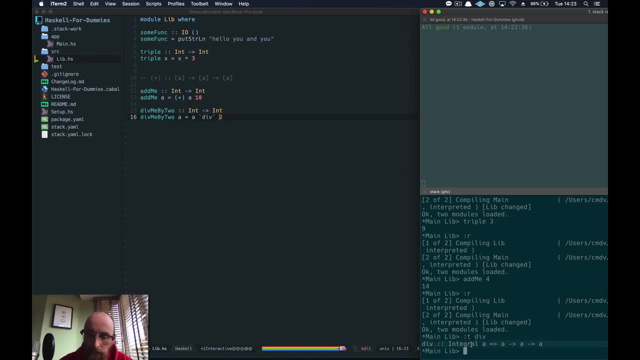 another a and returns us an: a. well, it's, and the a's are constrained to integral. but i'll explain what this little part is in a minute. let's ignore that. but for this instance you can see. so it's readable like this: so you'll do an a divided by two. so if we do div 10, nope, if we do div. 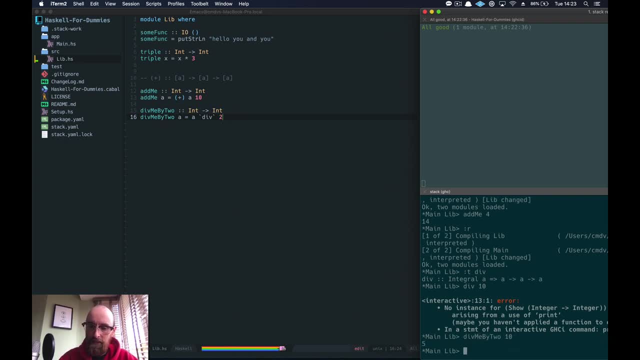 div me by two: 10, then that'll return us five, because it's doing, but when it's not in an invariable infix position to get the same result, you'd have to do it like this. so let's refresh that and we get the same results: five, okay. so that's what an infix is and you'll find that. 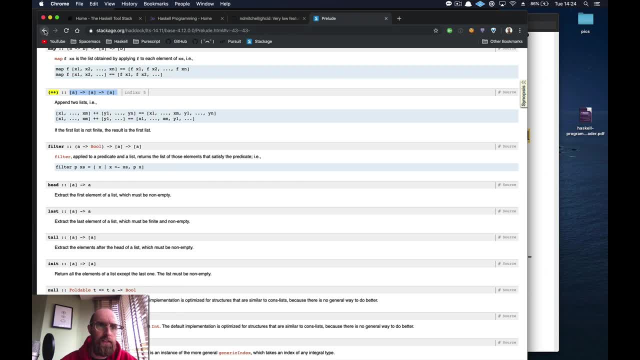 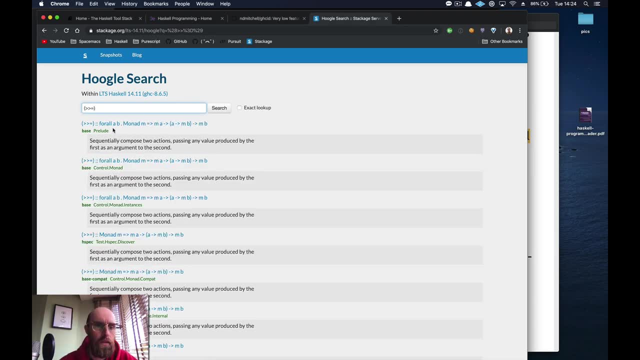 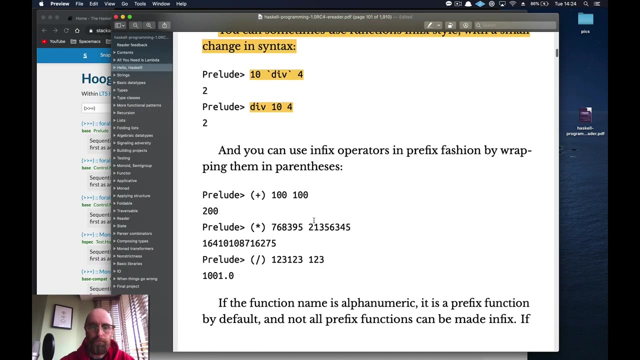 a lot of the times, if you are searching for something it's it can be easier to search for it in an infix like this. and there we go, so you can find bits and pieces in the infix, okay. so that's an example of that. and then we've got associativity and precedence, so it's much like 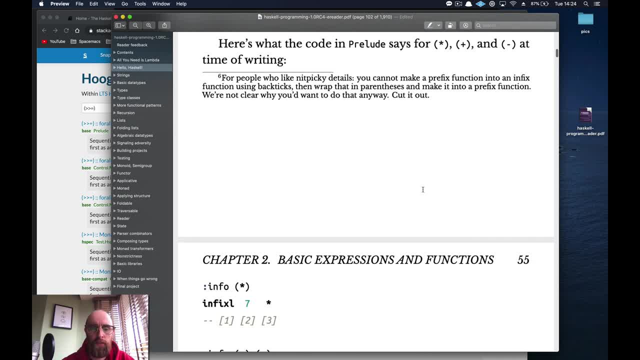 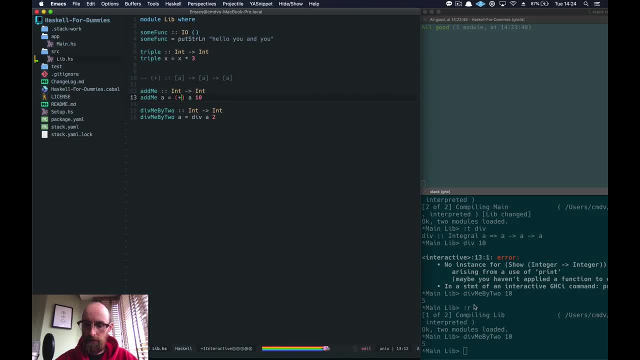 all other languages um things will take a specific associativity and to demonstrate that is you can find out the info. so let's type that in an rrepl. you can do shortcut i and we'll give it the infix. there we go. so it says it's an infix of seven. so we'll give it the infix of seven and we'll give it. 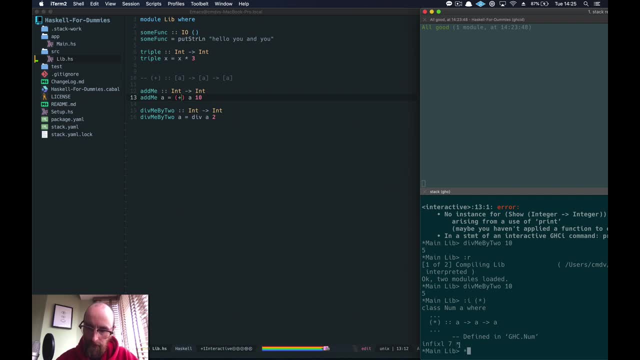 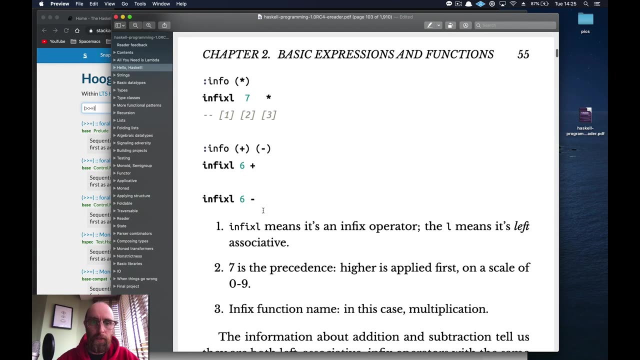 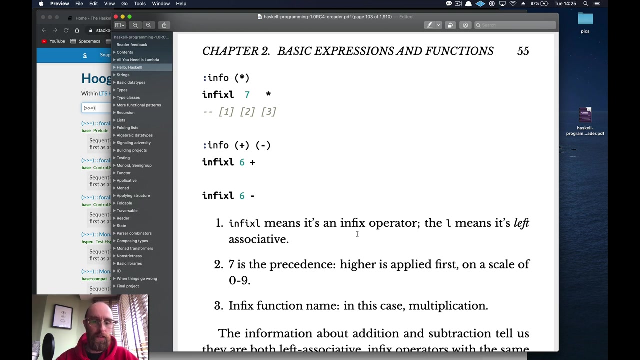 the infix of seven and that's the function name star. okay, so that's an infix of seven. infix l with seven, sorry, okay. so let's explain what the so the infix l means. it's an infix operator, so it's on it's left associative. the seven is a presence, so the higher is applied first. on a scale of 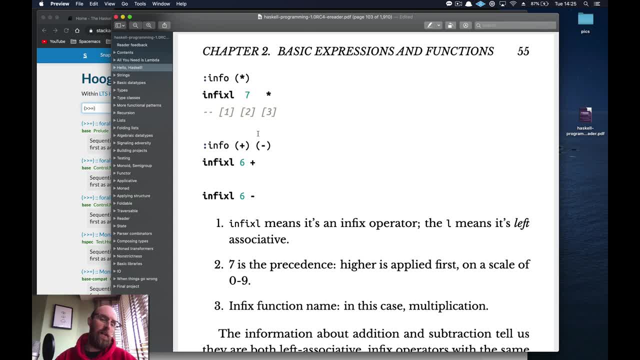 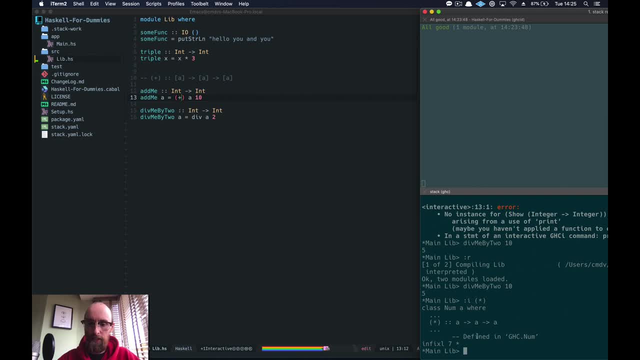 naught to nine. so sometimes you get infix l of one and then obviously seven to take presence of that and then that's the name. so the star would be a name. so if we do info of oops, if we do info of plus, then you'll see that's got an infix l of six, so that's got a lower precedence than star has. 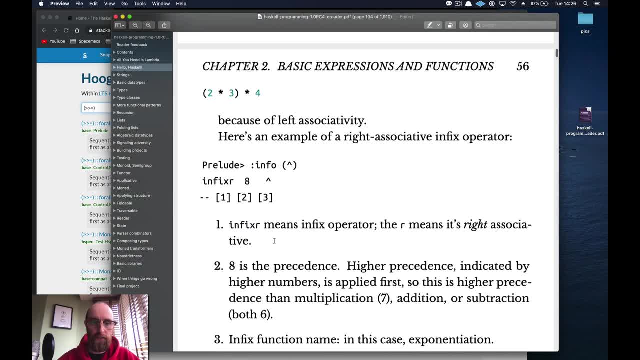 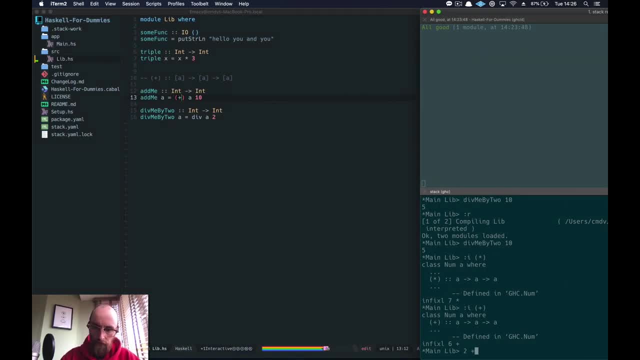 or times. so that explains what an infix is. i mean it does. you can demonstrate that by doing it straight in here. so two plus five times six is 32, but then if you were to do two plus two plus five times six, that equals 42.. so you can see what it's actually doing, because the star 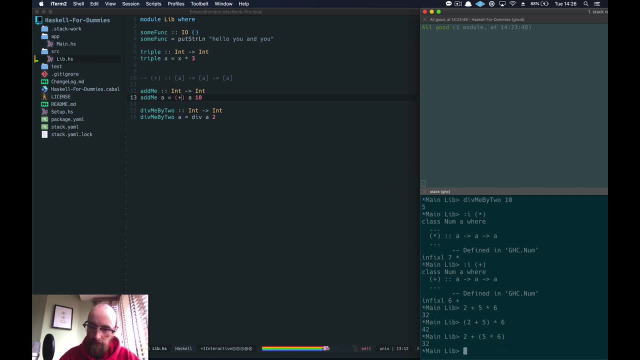 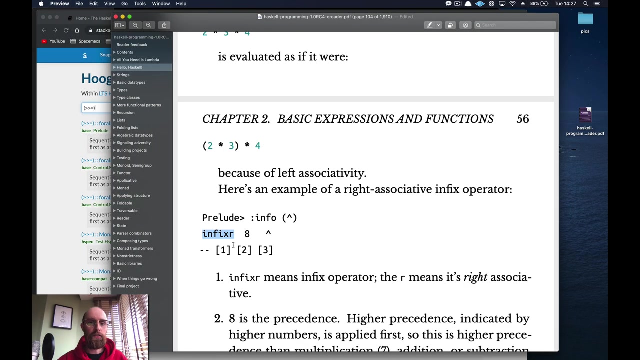 or the times is high precedence. it's actually combining it like this: okay, so that's, that's got higher, so that takes priority, and then the two. so it will bind those together and then it will take the results of those two and then add two to it, if you get to a point where you're going to make. 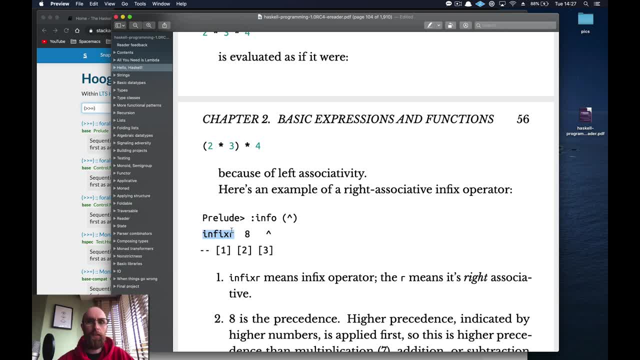 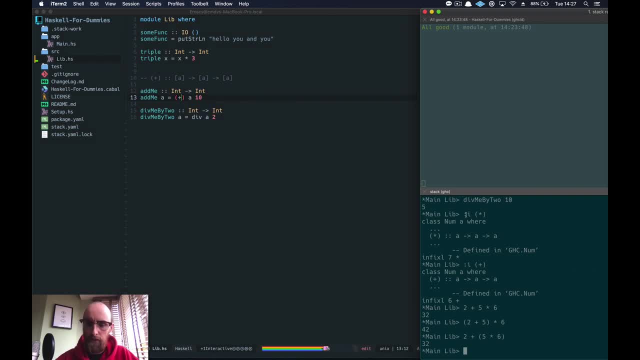 libraries, then this will be useful. but as for a beginner's point of view, it's just knowing that you can find out the precedence of something just by looking by info. so you know, if we did the i shortcut in i but info will work too, and then we can look at plus pass, for example. 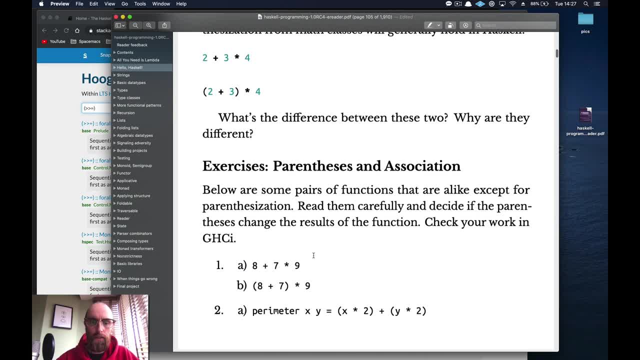 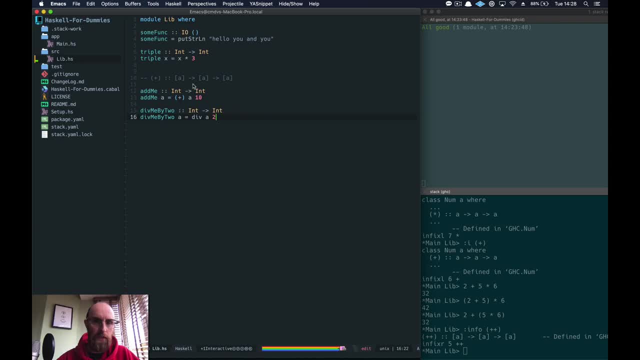 there you go. okay, so when we write values like this, it doesn't matter what all of these functions are set in, because ghc will load everything in the file at once. but then if you try and do the same in the repl, it does matter. um, it's going to be sort of one at a time. so if you're going, 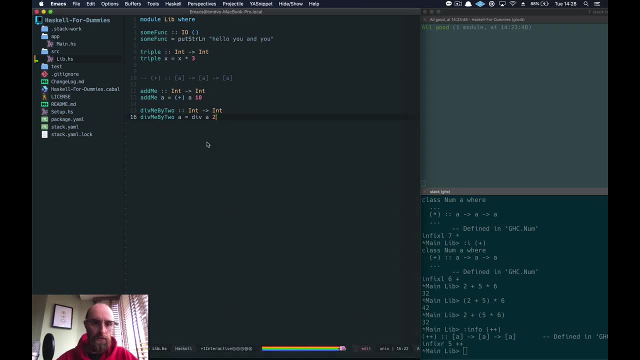 to declare a function. so let's have a little example quickly. um, okay, let's make a, create a function, func1, and that'd be int to int, and then func1: a, a plus. let's do a plus two, okay, and then let's do func2- oops. 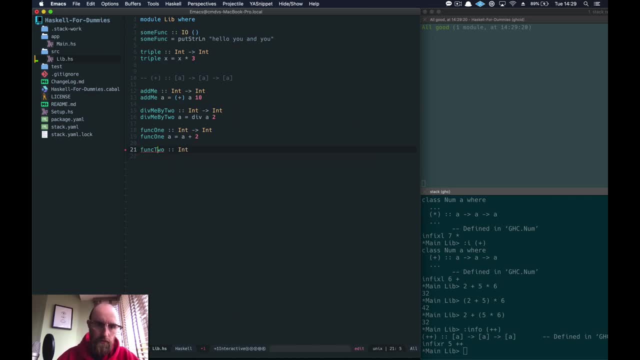 int, actually let's just call it two, and that would equal 12.. okay, so if i reload it here, actually let's make a third function, three, and that will just result us in an int when we call it, and that would be func1 and we'll pass it 2.. 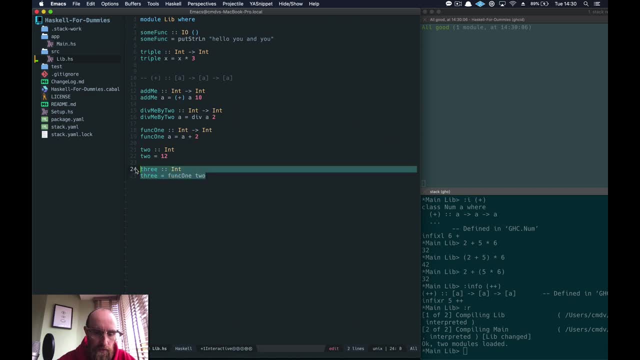 as you can see, let's- let's see how it works- actually put this in a different order for now, so we'll put that above these two, so it's clearly using something that's from below, and then we'll reload it and we'll call 3 and you'll see it'll. 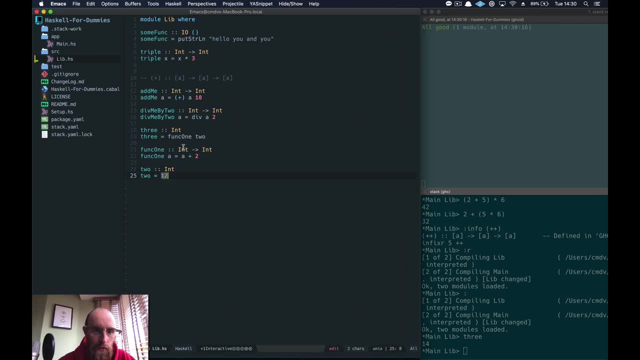 give us 14.. so that's. it takes the 2. we've passed the 2, which is 12, into func1, so that becomes 12. 12 plus 2 equals 14.. okay, but if we're to then do this inside the REPL and we're to try and do it, 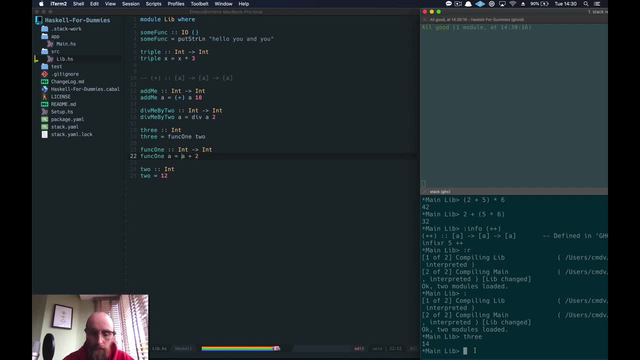 the same way. so let's say we do, let's make a function, so call it f1. actually we'll call f3 equals f1, f2. well, they're not in scope at the moment. there's nothing in scope, so it's not going to find them. they. 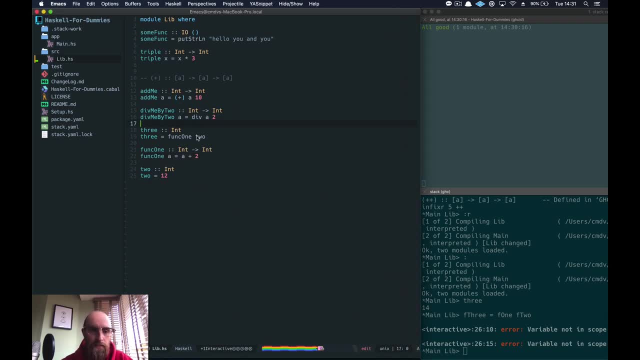 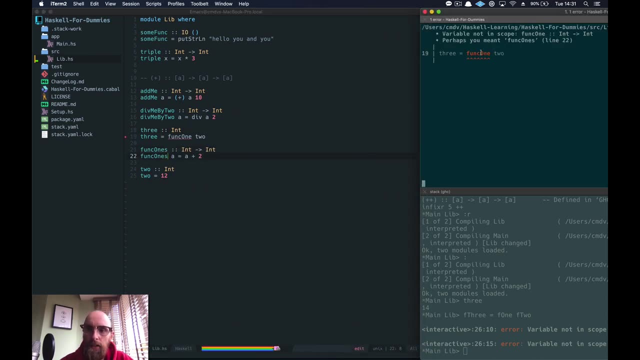 already have to exist to then be able to use them. but here, in essence, if those weren't there, if we were to call this ones, for example, save it. there we go. it's saying: i can't find func1, but in terms of its order it doesn't really matter, it's just the fact that it can't find a function. that doesn't. 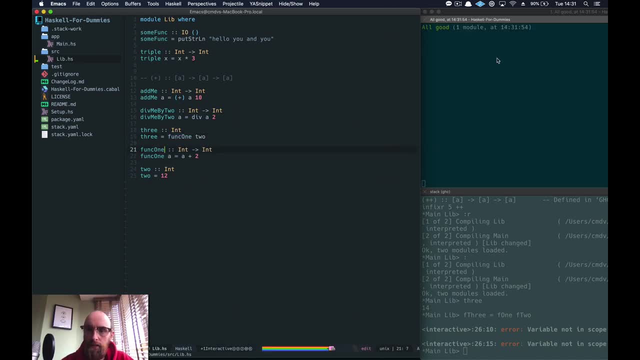 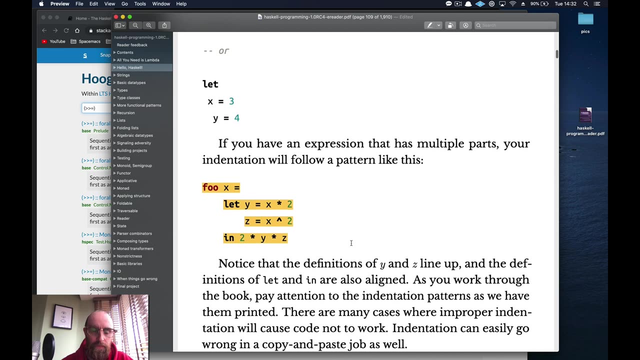 exist. that's the error we're getting, so we can save that again and that's back to all good. okay, so now we're gonna talk about a let, because sometimes you want to declare things that are gonna stay inside of a function. you don't want it to be outside of that function, so we can do it like this. so let's take 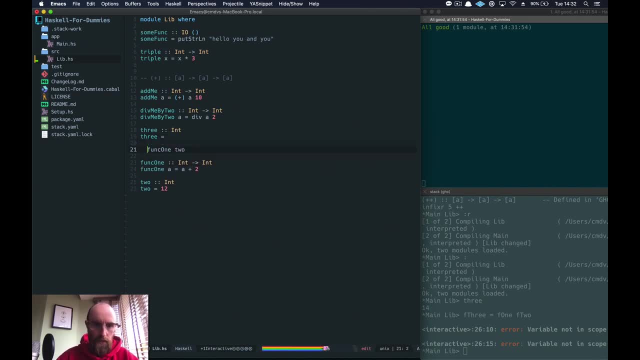 this free apart and we're gonna do it like this. so we'll do a let and we'll call it func1. takes an a and does a plus two. then you've declared a let block. you want to align with the function above, so we'll do a func. 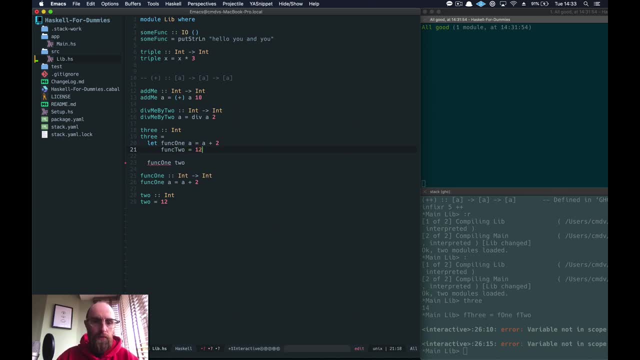 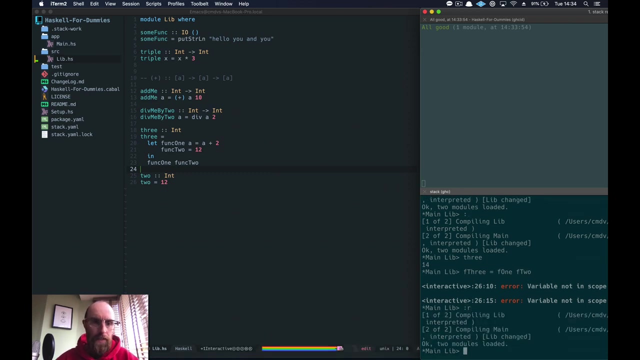 two, and that was just to equal twelve. and then you want to use a keyword in. what i'll do is: i'll delete that. so, as you can see right, we'll reload it and let's try and use func one, twelve. it's not in scope, so this func one because we've declared it. 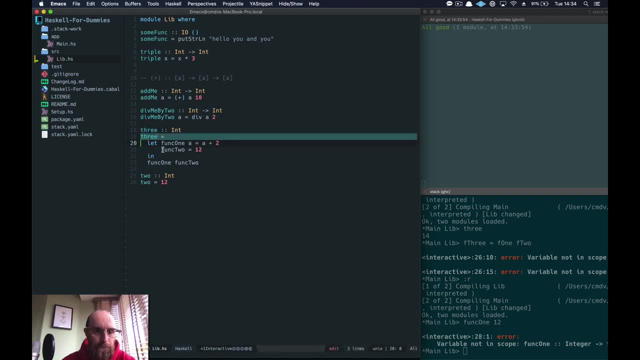 here it's only available from within three and then you can see we use it here the same as func2, but if we called three itself, then that'll work. so you can see how in the encapsulation is sticking within and you're doing let in and that's the keywords. you can see. oh, 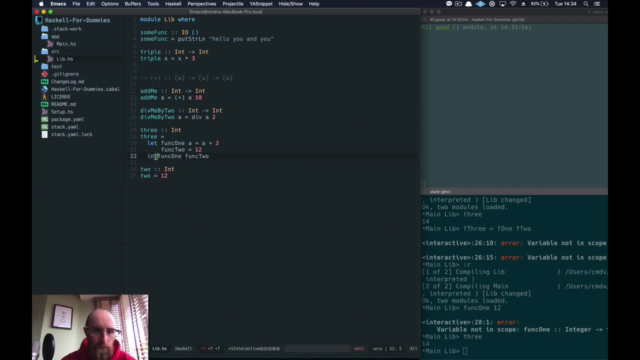 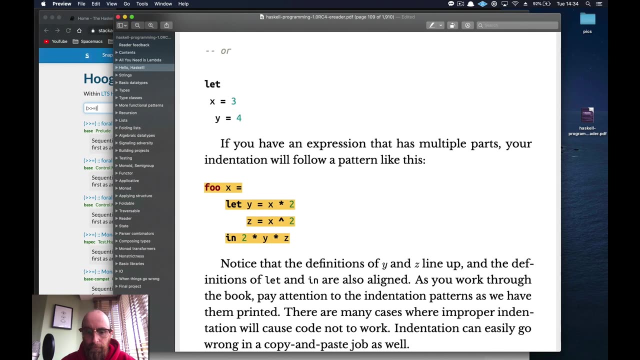 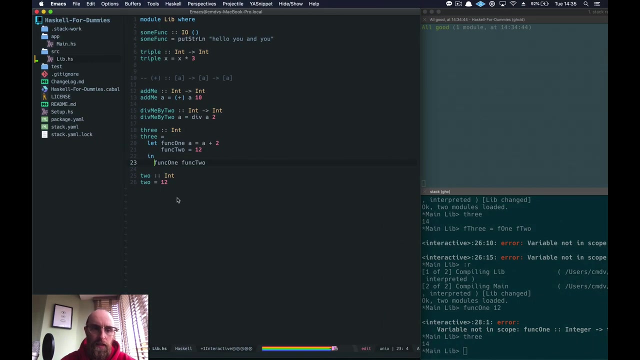 i mean, they've even put in like this, but you can have it both ways, it just depends stylistically how you like it. oh, like that, yeah, okay, this is showing you a declaration and something like that would break. so let's say it was x equals 10 times. 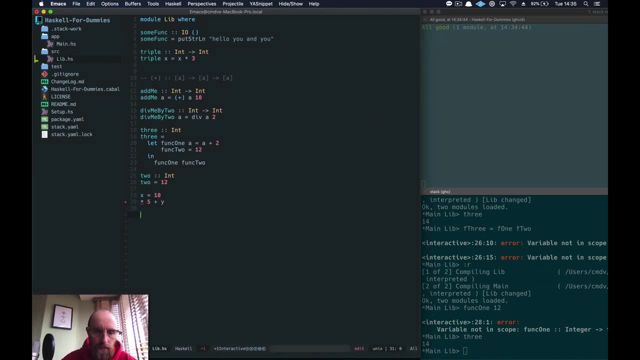 five plus y, and then y equals, y equals 10, and then let's have my result equals. let's change a little bit x plus y and we'll save it. and it's going to complain straight away saying, well, i've not been able to pass it, there's something wrong here and that's not going to be a problem. but what you've done is you've. 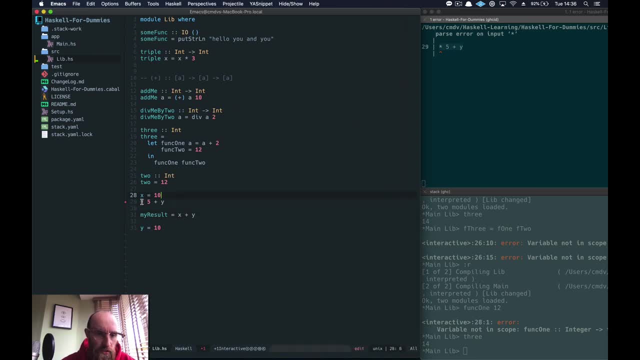 here. so if you want to declare a function as soon as you go on the new line and you have it- the same level as the name, so the same indentation as the name- then this is going to be a pass error. it's just this could be somewhere here, you see. so it's a totally different function right now it's taking 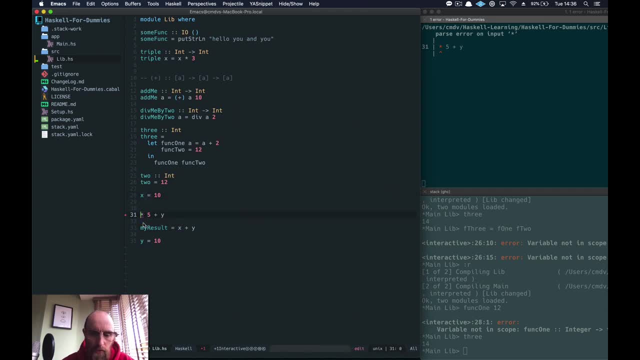 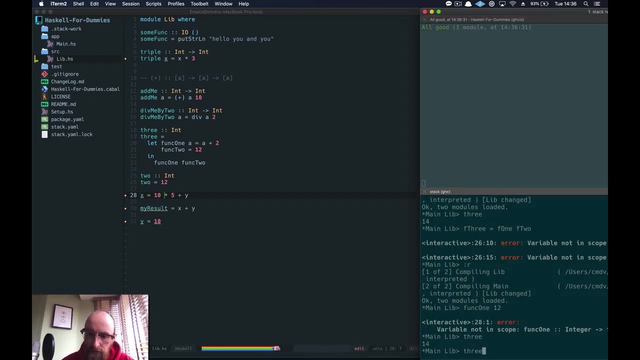 this as a function and it's not finding an equal. so it's going well, what's going on? but if we were to do it like this, then that would pass. you see, and then if we're to do, and if we're to reload that, and then we do, my result, and it'll be 70, 10 times 5 plus y is 60, and then 60 plus 10 is 70. 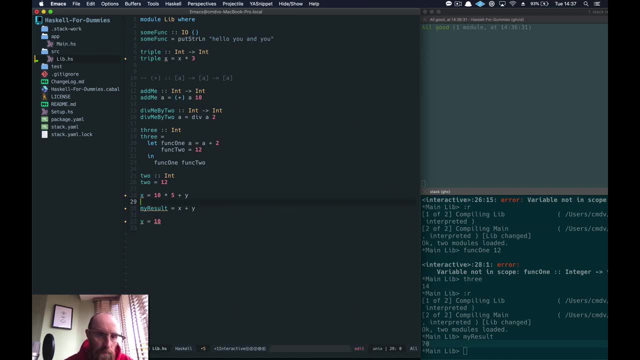 that's that part. so you've got to be careful with your indentation. you can do this. that's fine. you've got to be careful with your indentation. you can do this. that's fine. that's fine. that's fine. i mean, that's not very pretty, but it can count, okay. one thing i've not. 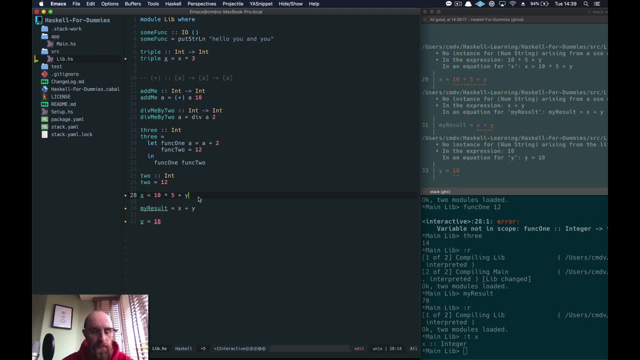 explained is how ghc automatically infers types for you, and there's a more technical word for it, but i'll demonstrate what i mean. okay, so if we find out the type of x and that'll give us an integer, so it's saying that x is an integer. 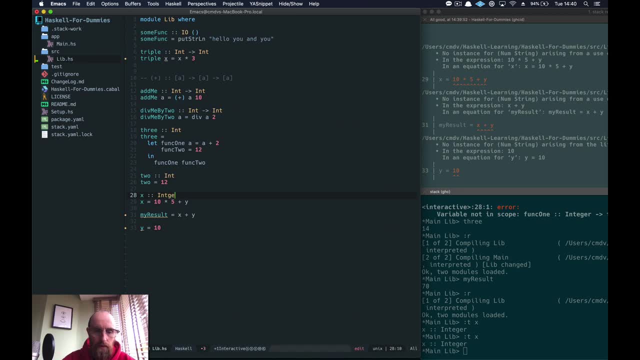 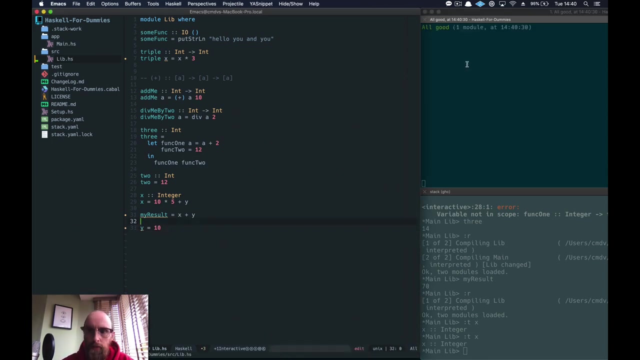 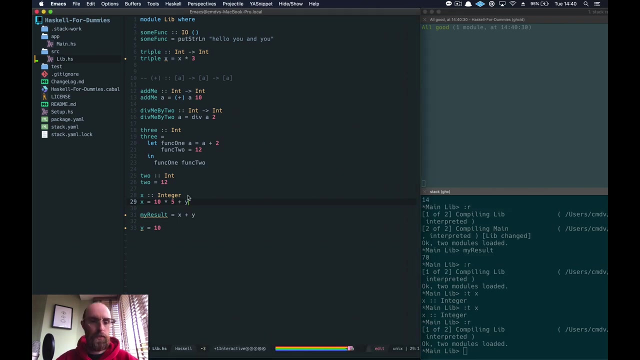 so it's saying that x is an integer. let's do that, okay. okay, i'm just doing that. so it really goes up. there didn't seem to jump. so it's automatically inferring what our types should be. but just remember, you don't necessarily need to give. 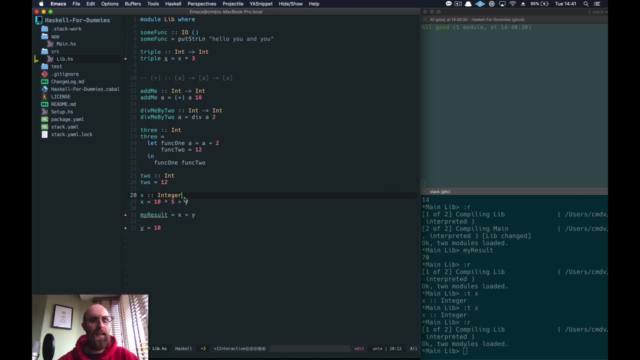 types. you're leaving yourself open to the fact that you don't necessarily need to give types. you're leaving yourself open to the fact that you don't necessarily need to give types to errors if you're not going to declare the types of something because ghc will infer them for you. but what if it infers into? 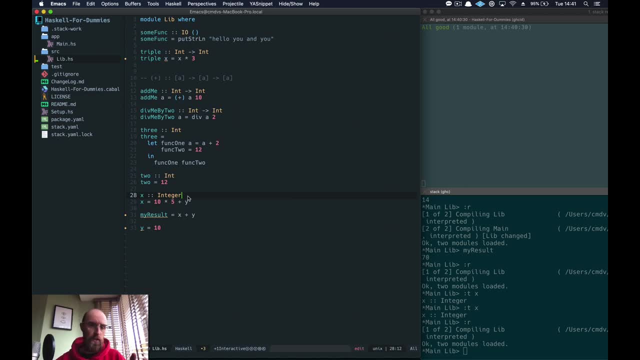 an incorrect type and then, for some reason, you've got two types that don't match and you're not. you expect them to match, and then you're opening yourself to a whole load of trouble. what we tend to do is give everything types, so like that, we you know, there's no mistake. 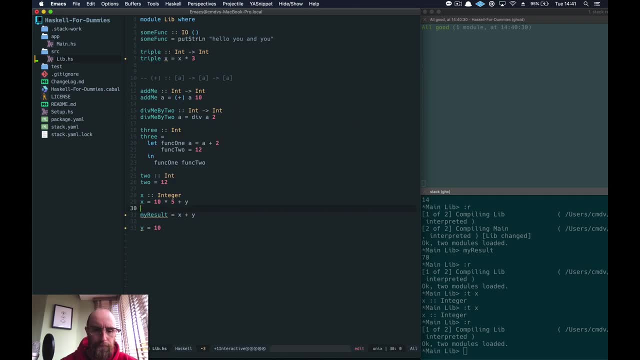 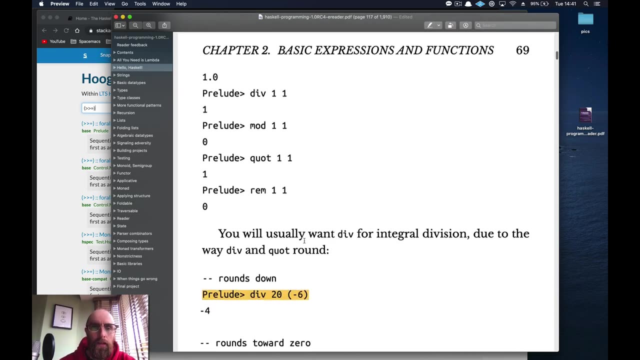 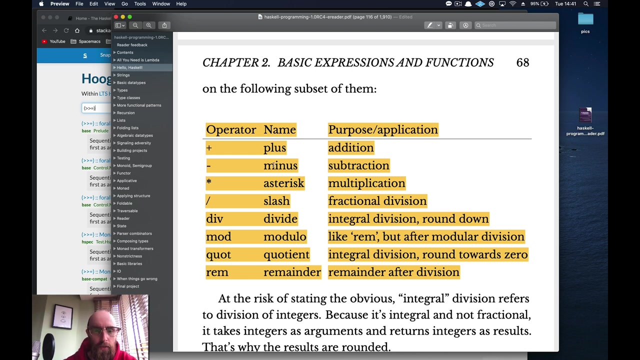 the compiler has a really good idea of what values should be okay. so if we go to the next part, oh, here we go. okay. so that's just our operators and what they do. so obviously the plus is plus, addition, minus is minus, abstraction multiplication. for the asterix, i call it star asterix slash. 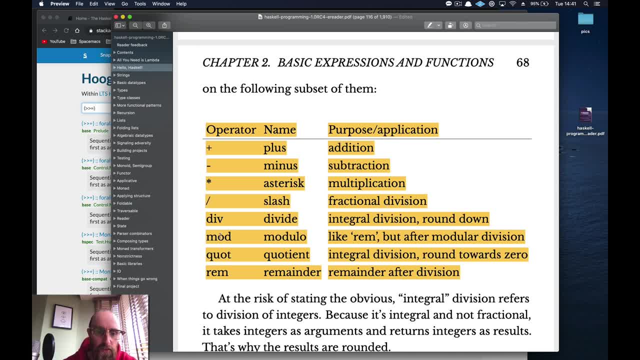 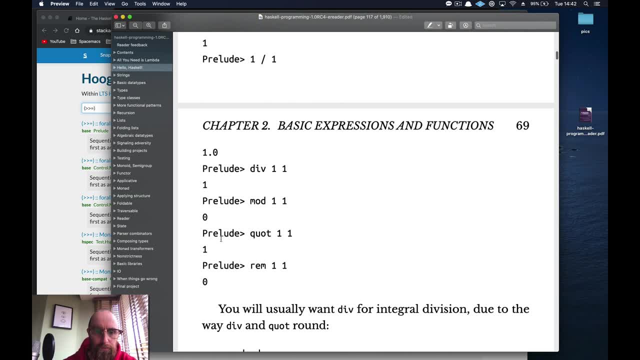 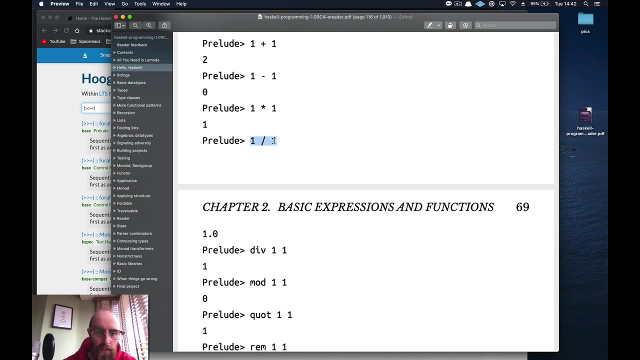 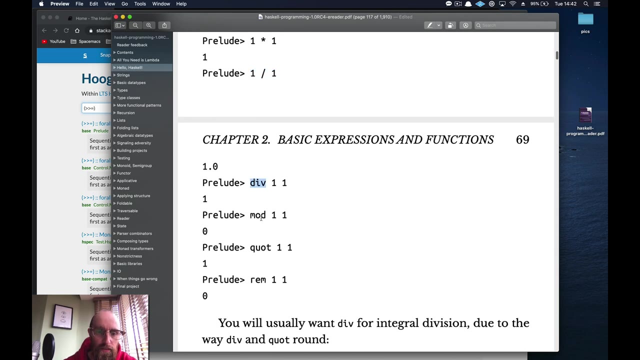 fractional division divide, whereas there's div, mod, quote and remainder, and we'll go into those. actually, let's have a look so we know how obviously class works, how times works, how how slash works. so that's a fractional division and then we played with that modulus or mod. 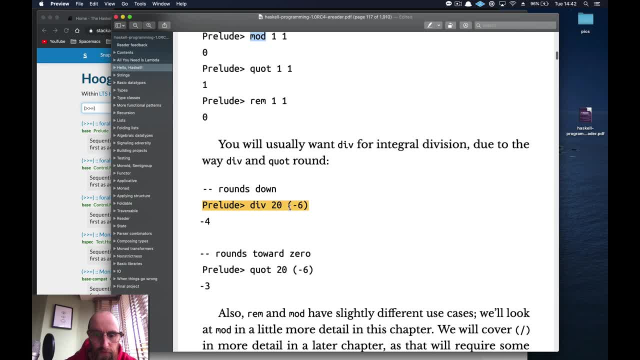 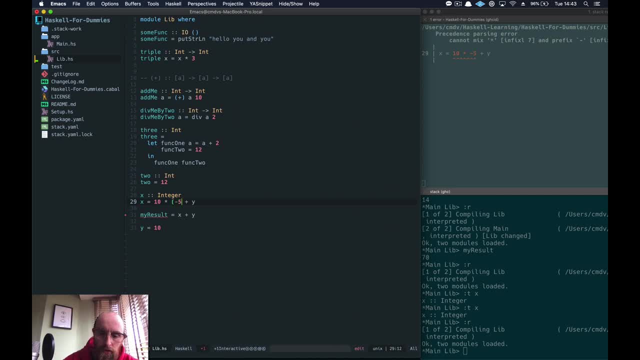 quote and remainder aha. another thing to remember: it's because we can't simply do that. you have to make sure you wrap it. instructions, because no notes for the second step is significant. they built because we think over them and then over there, a million notes is not any reason. it's not important for them to use them. we can't just simply implement a recursive formula. that's totally nonsense and we've got to make sure you wrap it. so if you want to act as if it's important in the certain ways that I'm using it, I show you aàoama and let me leave you with your statements and I'll ask you toiendokou in the second question. 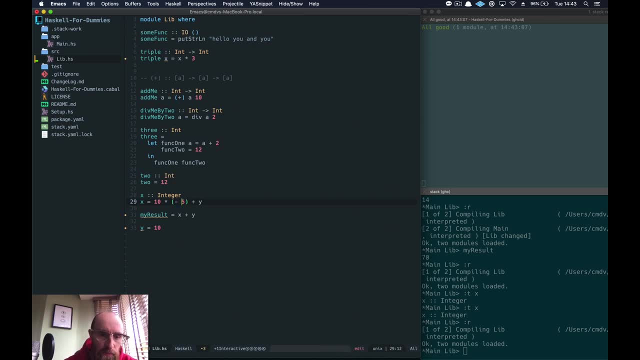 flower. there we go, thank you, because if you think about it, it infers that to be minus and if we look at the type of minus, see it expects two values. but then if we're just putting it in there, it's saying, okay, well, i want the first value, and then i want the second value, but then you're giving it this as a second. 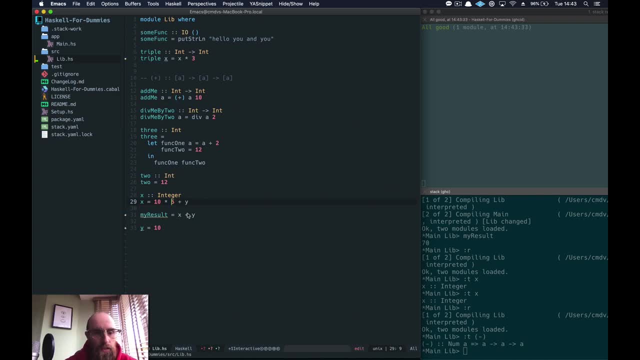 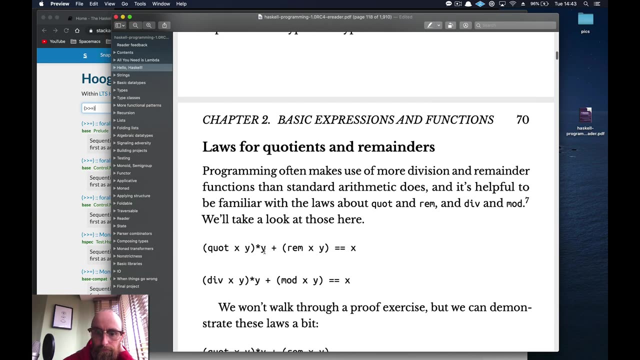 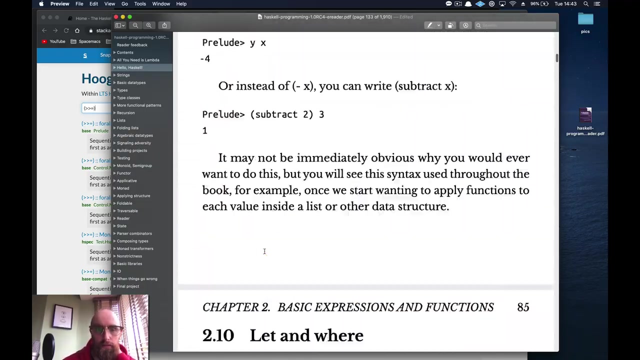 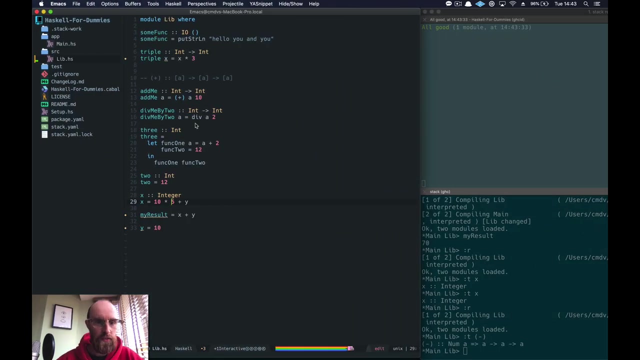 value and it's just getting confused. so remember, you want to make sure if you do a minus is to wrap it around and then to make it really implicit what it's going to be. okay, we'll skip by this. aha, okay, so we had a little look at let before. this was quite good. here's our let. 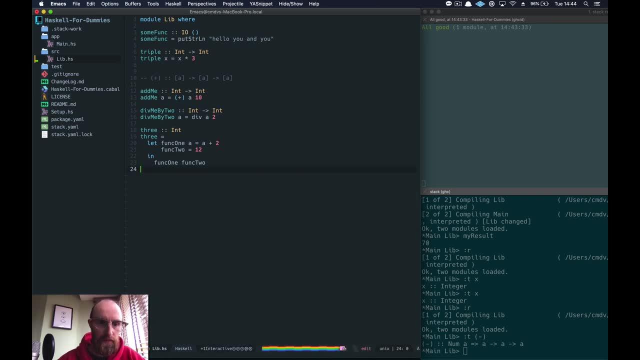 okay, i'm going to delete those guys because they're probably not needed, and let's make a where func, where's our func, and this can just return us an int. and then there's where func, and that equals. let's do, um, yeah, f1 plus f2. 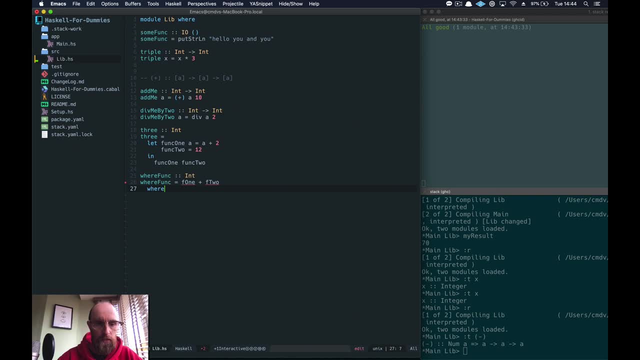 make sure you tab it across, or i don't do it by two spaces, and then you can do this. so f1 equals 12, f2 equals 10.. okay, let's have a look what happens here. we'll reload that and we'll do our where func. 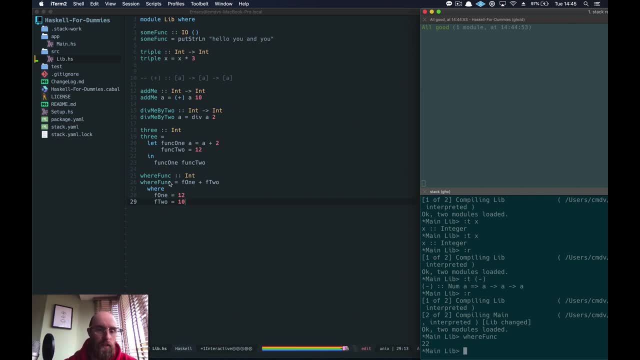 22.. so we're doing: 12 plus 10 is 22.. so look what happens here then. so we're again much like the let you know. let's have a little. look f1: nothing, it's not in scope, okay. so it's again. it's encapsulating. 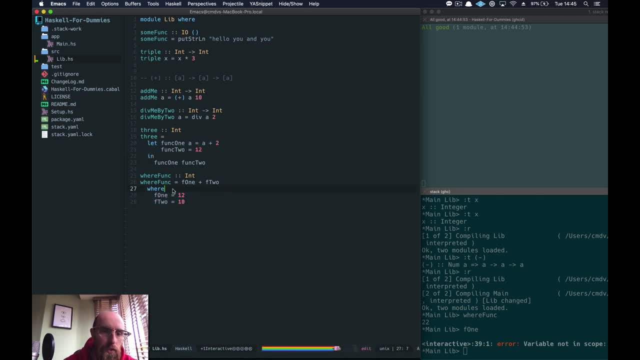 things. it's the same version of this, but what you end up doing is declaring your functions below, within the actual function itself, and then using it above, so what this is called here is aware clause. so once it's gone past this section, whoop. now you're within the where clause, the other useful. 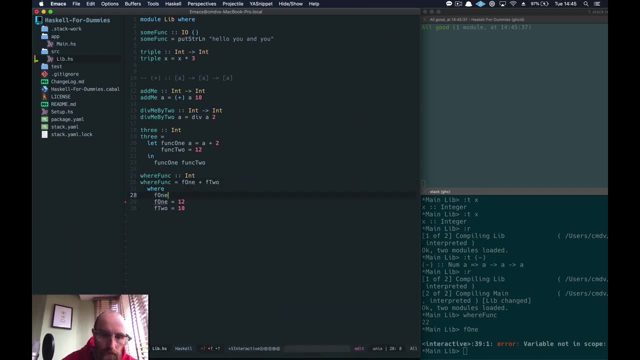 thing you can do with where clause is this: you can give it type definition f2 and that's an int like that. so i mean so a lot of times you'll find if it's functions that aren't really going to be usable or you don't want them to be accessible outside, a lot of this will. 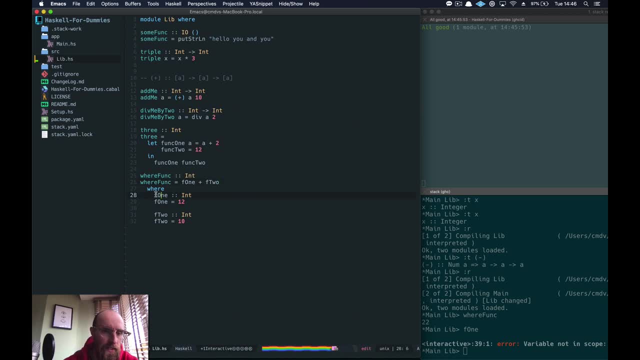 happen in here. a great thing about this is you're making sure that these are scoped to only inside of where func and then you're not exposing them outside. so it's very similar to this, but it's inside and you can also give them type definitions. so i mean, if i try and give this a type definition, 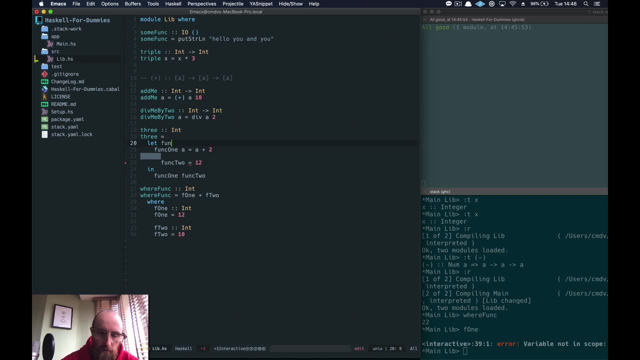 it won't work, which i'll demonstrate. func- whoops. one is an int. okay, there we go. so it's just not recognizing it. it expects just it to be a function. so let can be nice. you're going to do like little tiny things. you know functions, you, you know what you expect them to be. but for readability, it's nice to have the ability. 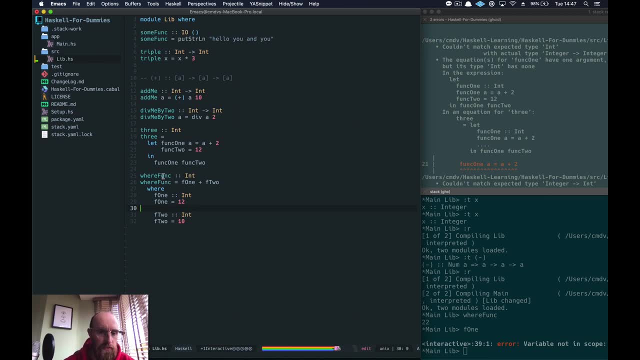 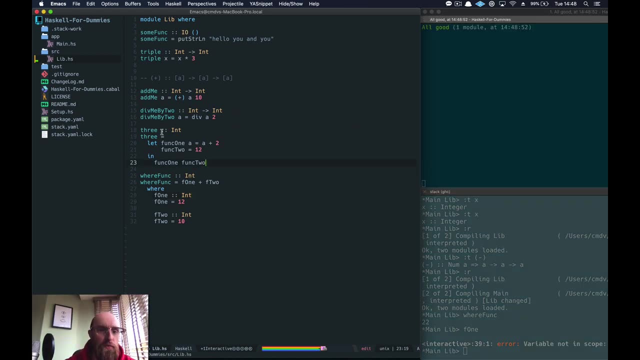 to do this. so then, if you've got more complex functions that you don't want to be outside of this scope, then at least you can give it a type and you know what for what to expect. okay, another cool thing with both of these is if you declare something up here, so this is an extra value, that's. 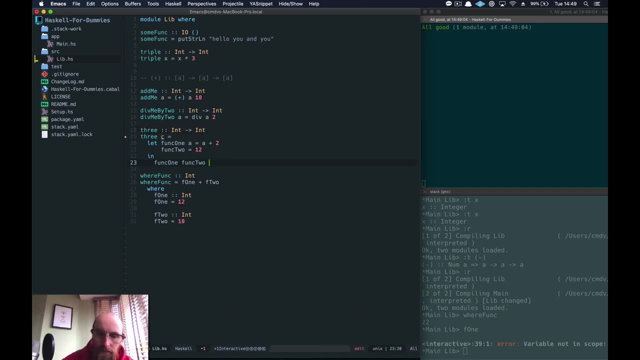 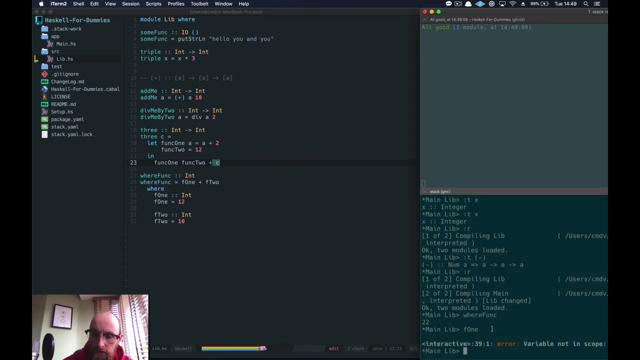 going to come into our function and we can, so we're going to add the results of them to with a c. okay, so that'll work. let's have a little try. so that's 3, and we're going to give it a value of 4, and that'll give us 18, so it's 12. 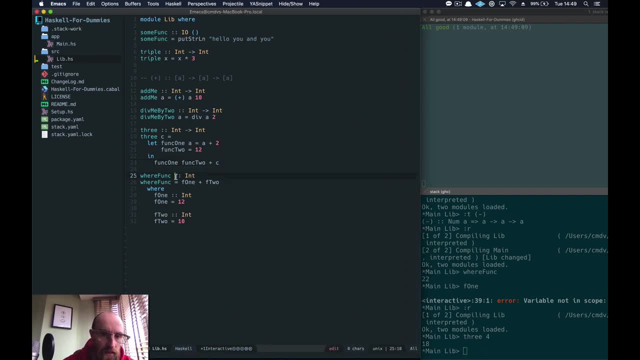 plus 2 is 14, plus 4 is 18, and if we try and do the same here. so it takes an int, oops, returns an int, and we'll give it that as c and then we'll do 12 plus c. there we go, we'll reload that and we'll do where funk. 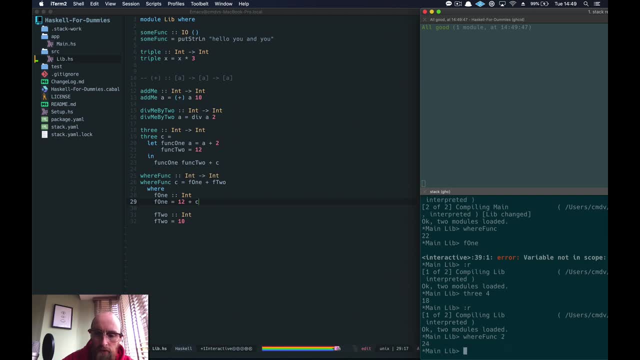 and we'll give that a 2.. it'll be 24.. 12 plus 2 is 14 plus 10 is 24.. okay, so we've still got access over here. but if we try this, let b equals 11 in like this. okay, so we've got a b that's not being used, and then 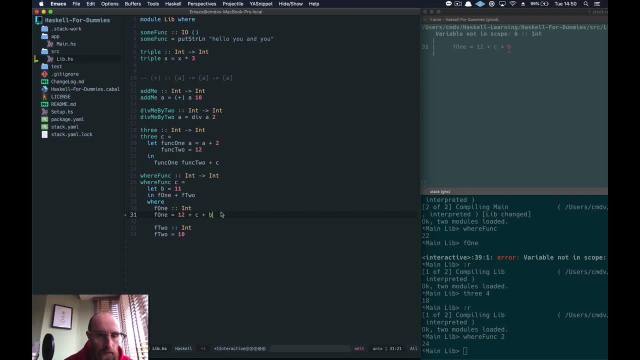 we'll try and refer to our b. it's not going to find it okay. so what you've got to keep in mind is where clauses can access um top level inputs, but it can't access anything that's declared inside the function. but this can. so you see. so you see how it's accessing these two functions. they're. 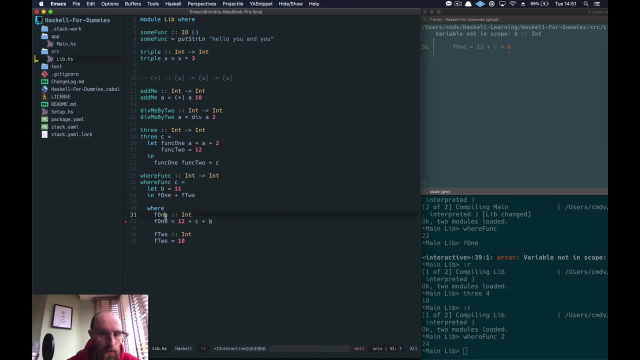 within. but this doesn't okay. so once it's in a, where clause, anything that's declared inside of where function ie b, it's not going to find it. it's going to say, well, i haven't got a, b in scope because these essentially act as little functions, but the only access they've got is up. 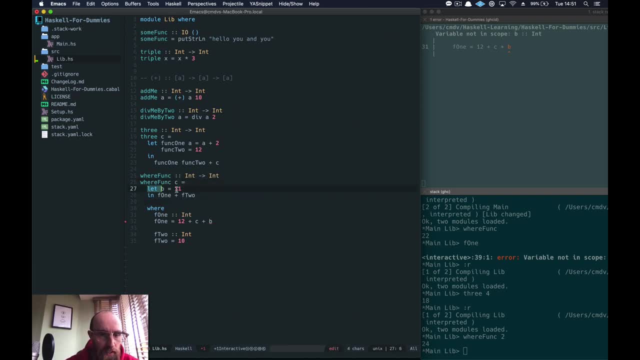 here. that's the only access they've got. they don't have any access down here. so here we're essentially doing the same as this, but we're then defining our functions. these two functions um to exist in the where clause, and then we're able to define the types for them. okay, so i've. 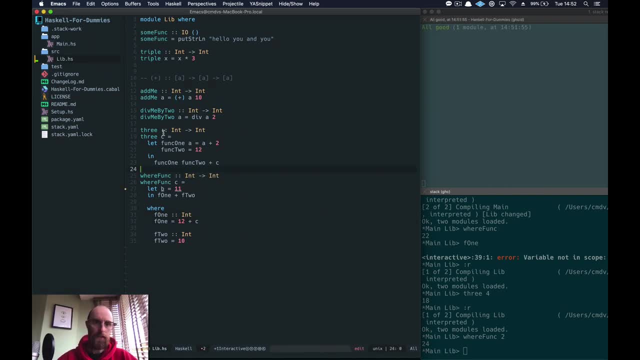 demonstrated that right. well, i think that's potentially enough for today. so i've explained a little bit more about functions, how they're laid out and what you can do with them. we've had a little diving with a type declaration. we've not quite explained what this is, but that'll come um, so you. 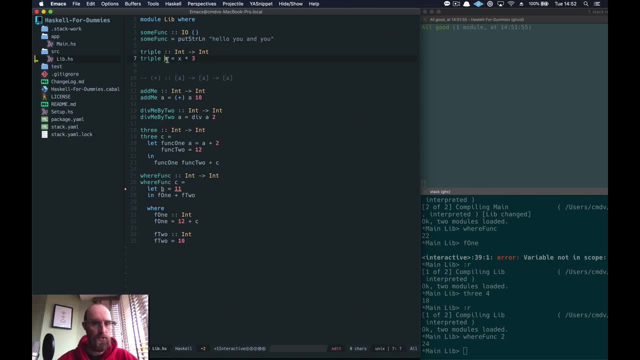 know we have something, we expect it to be an input which sits on the left, then we give it an equal and then an x plus three. that's quite understandable. here's the same. and then we also explained. you know the infix operator, so you can infix things, or, if you wanted, you could have him in here. 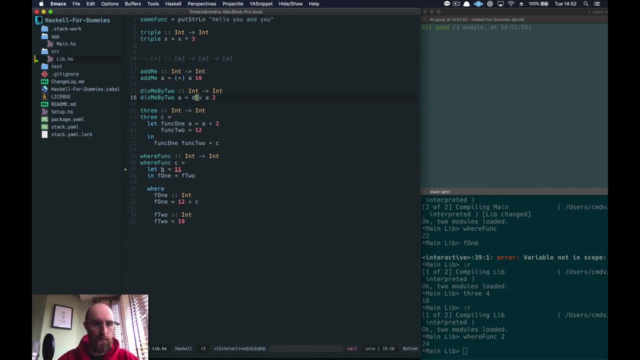 obviously you take the one away. uh, same with a div. the ones that are worded tend to be in fixed like: so okay, uh, we've. and then we explain what infix is in terms of like it's, it's a fix l and in terms of the number it can be. then we went into a let function, so you have to use. 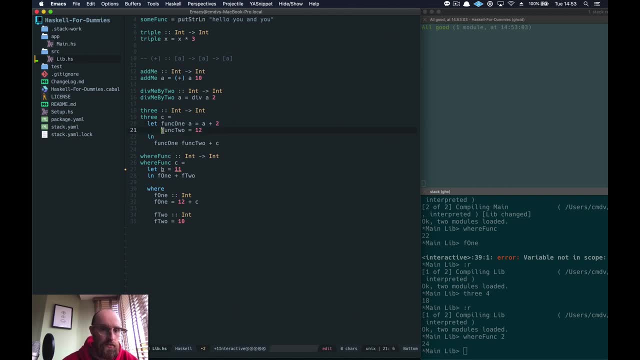 a keyword. let you declare a name of a function. you can have multiple functions if you want. you can keep going, but then at the end, when you want to actually go into the body, you have to do in. okay, so you do let in, and then we're using anything that's above. 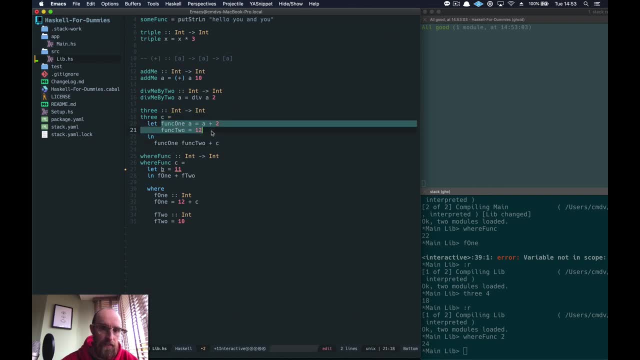 to do that. there we can get scope to here and here, but when using a where clause, it's very similar, but we don't get access to anything that's in the body. so here we're able to use anything that's below. so any of these two functions, but if you're going to want to pass it,